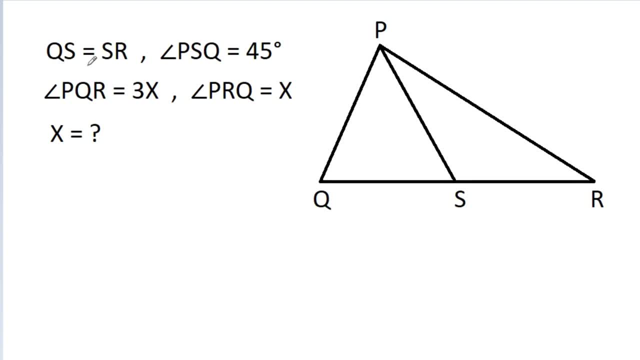 In this video we have given that Qs is equal to Sr. So Qs is equal to Sr and angle Psq is equal to 45 degree. This angle is 45 degree And angle Pqr is 3x and angle Prq is x. So 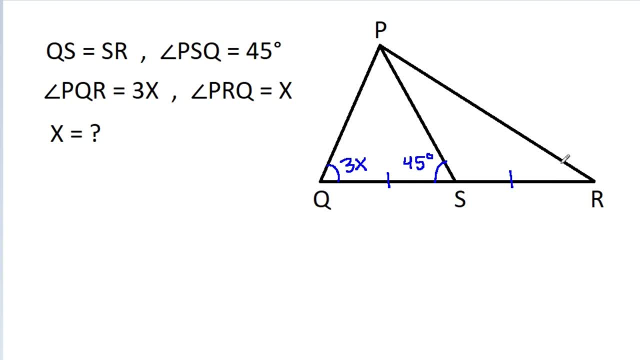 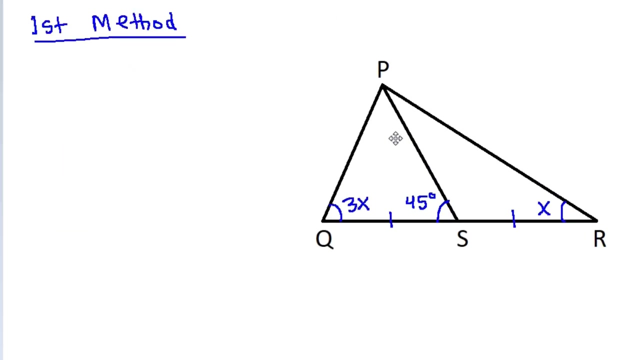 this angle is 3x and this angle is x And we have to find the value of x. So the first method Here, Psq, Sq by Qs Award to, and then we have corrected calculation of QS- is equal to SR and in any triangle of side length A, B and C, and this angle is A, this 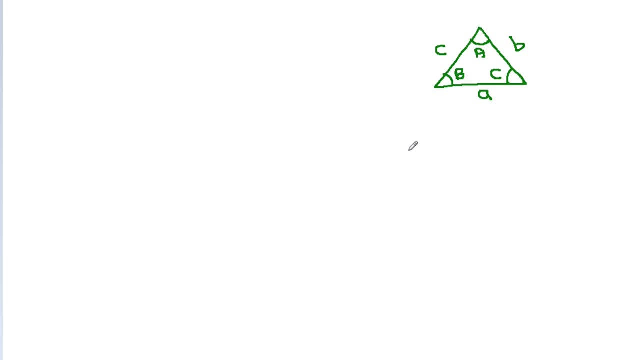 angle is B and this angle is C, then A by sine A is equal to B by sine B, is equal to C by sine C, and we have: A by sine A is equal to B by sine B. That means A by B is equal to sine A by sine B. 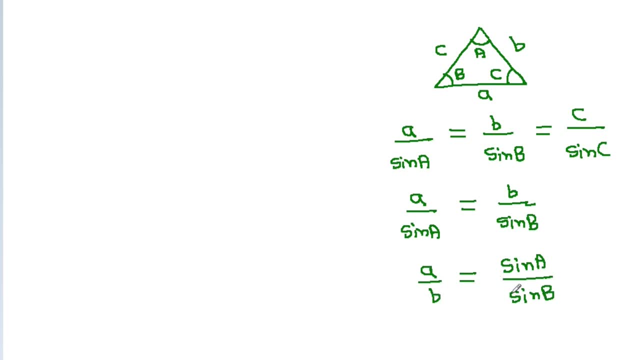 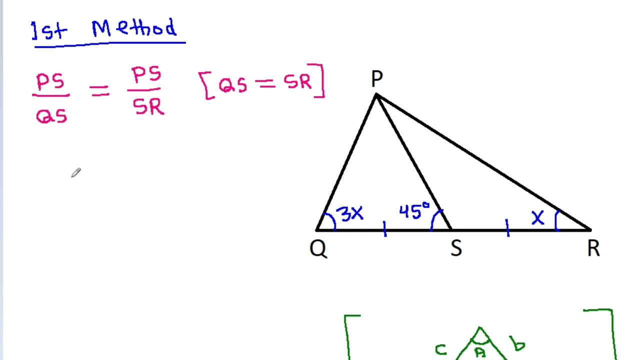 That means ratio of side length is equal to ratio of opposite angle. So here PS by QS will be equal to A by sine, A by sine B. That means A by sine B is equal to A. A by sine A by sine X by sin X by theta. 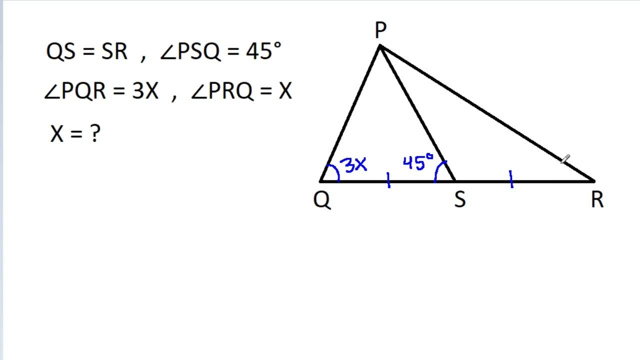 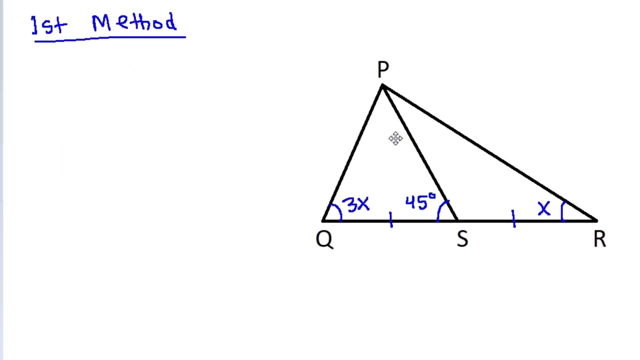 this angle is 3x and this angle is x And we have to find the value of x. So the first method Here: Ps by Qs will be equal to Ps by Sr, because Qs will be closer to Sr than Sr, so Prq will be closer to Sr. lasiados method is my first. 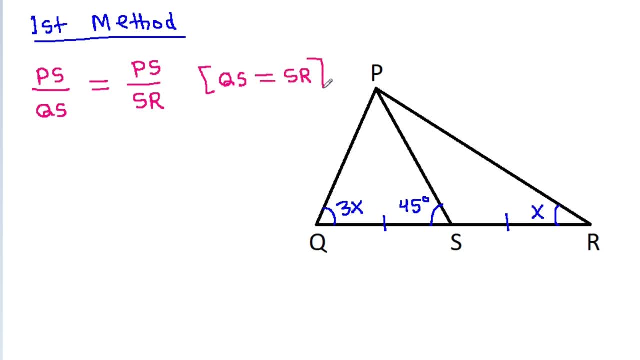 QS is equal to SR And in any triangle of side length, A, B and C and this angle is A, this angle is B and this angle is C. Then A by sin A is equal to B by sin B is equal to C by sin C, And we have A by sin A is equal to B by sin B. 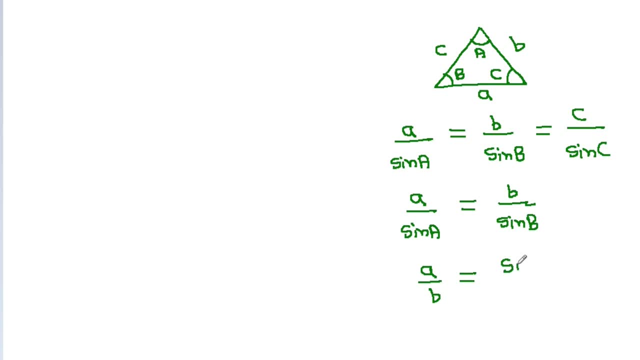 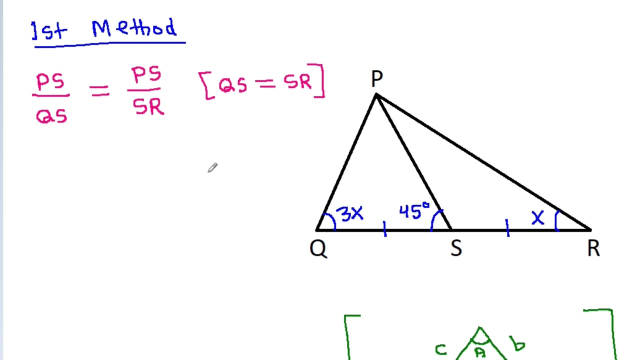 That means A by B is equal to sin A by sin B. That means ratio of side length is equal to ratio of opposite angle. So here PS by QS will be equal to A by sin A by sin B. So here PS by QS will be equal to A by sin A by sin B. So here PS by QS will be equal to. 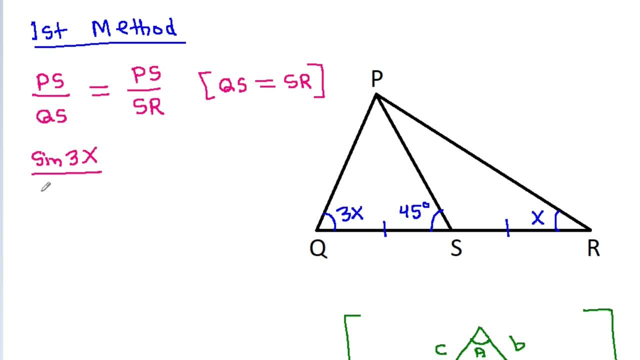 sin 3x by sin A. Suppose this angle is A and this angle is beta, It is equal to, and PS by SR will be sin x by sin beta. And in triangle- Pinterest triangle- PX by B is equal to A by sin B. 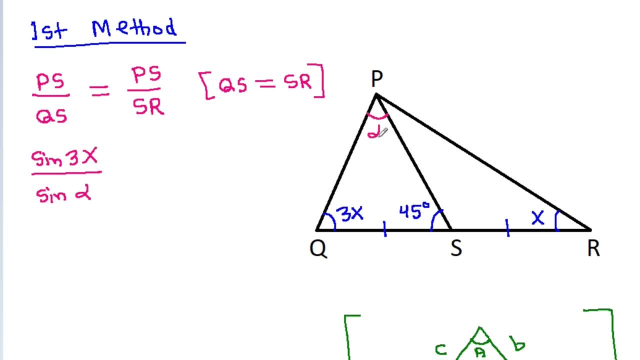 And P minus P is equal to A by sine 2ega, A by beta, by sine 3egs, by sin alpha. Suppose this angle is alpha and this angle is beta. It's equal to. and P s by SR will be sine X by sin beta. 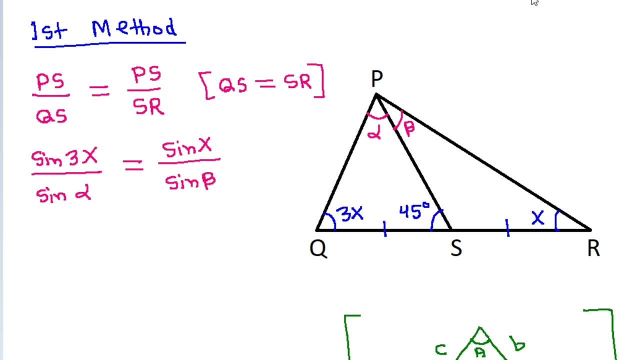 And inter angle P gets equal to Belungen and this angle also total. Listen properly, True or false. True PQS alpha plus 3x plus 45 degree, it will be equal to 180 degree. That means alpha is equal to 180 degree minus 3x plus 45 degree and this angle will be 135. 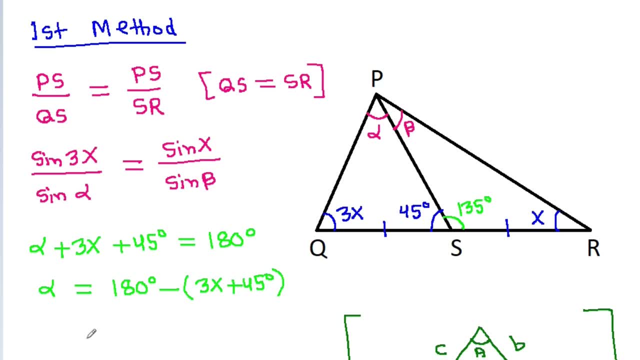 degree, So Close joint Laurke aimed angle. so interior angle PSR is equal to negative van. That means alpha is equal to 180 degree minus 3x plus 45 degree and this angle will be 135 degree. So intermediate angle PSR is equals to negative van碧. W would be 135 degree. 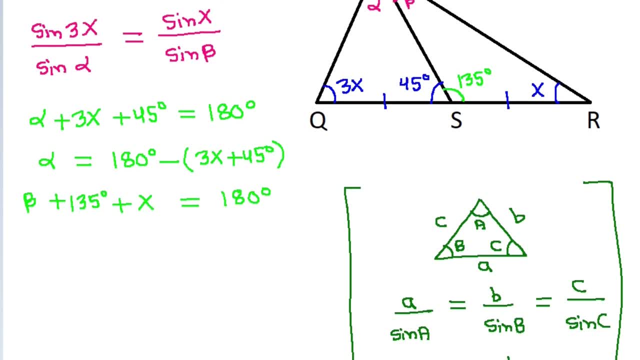 180 degree, so beta will be equal to 180 degree minus 135 degree is 45 degree minus x, so sine 3x by sine, and alpha is 180 degree minus 3x plus 45 degree is equal to sine x by sine. 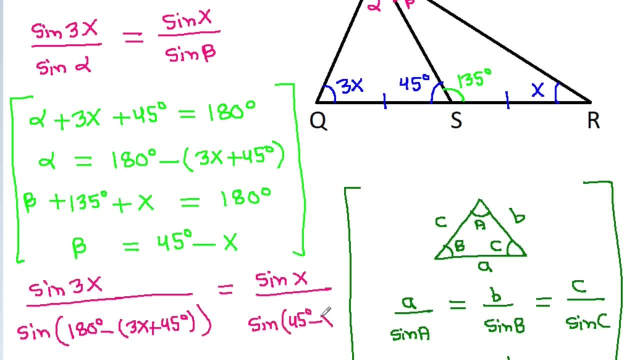 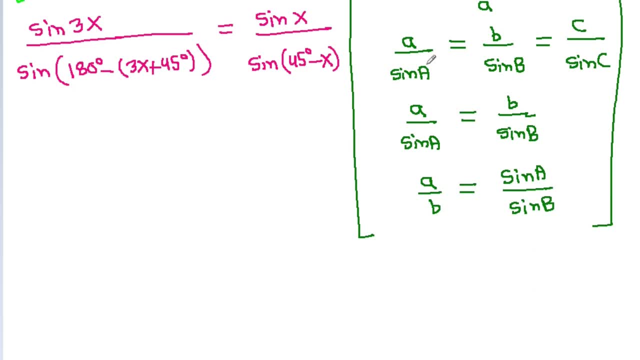 and beta is 45 degree minus x and sin 180 degree minus theta is equal to sin theta. So it is sin 3x by sin 3x plus 45 degree is equal to sin x by sin 45 degree minus x. And if we cross multiply, then sin 3x by sin 3x is equal to sin 3x plus 45 degree minus. 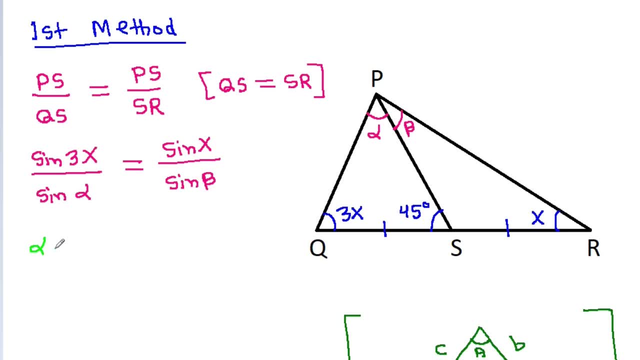 PX by B is equal to A. by sin P, Qs, alpha plus 3x plus 45 degree, it will be equal to 180 degree. That means alpha is equal to 180 degree minus 3x plus 45 degree and this angle will be 135 degree. So 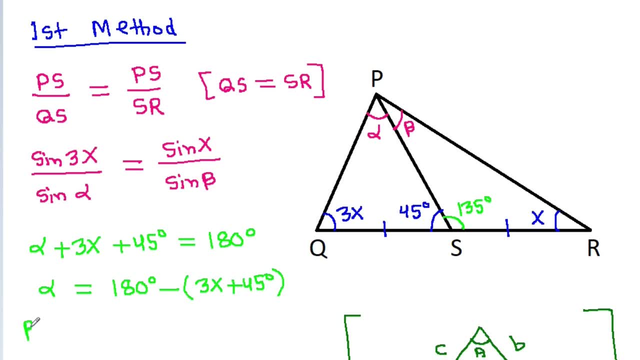 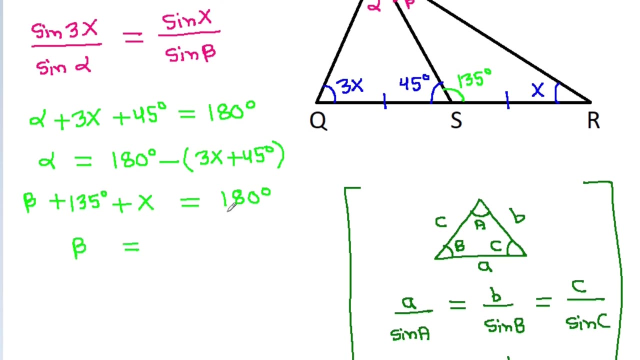 inter-angle PSR: beta plus 135 degree plus x will be 180 degree, So So beta will be equal to 180 degree minus 135 degree is 45 degree minus x. So sin 3x by sin and alpha is 180 degree minus 3x plus 45 degree is equal to sin x by sin. 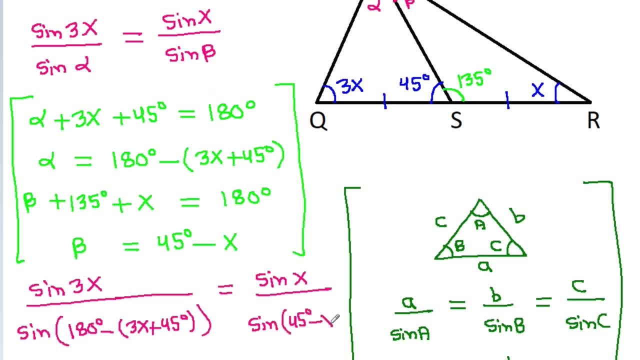 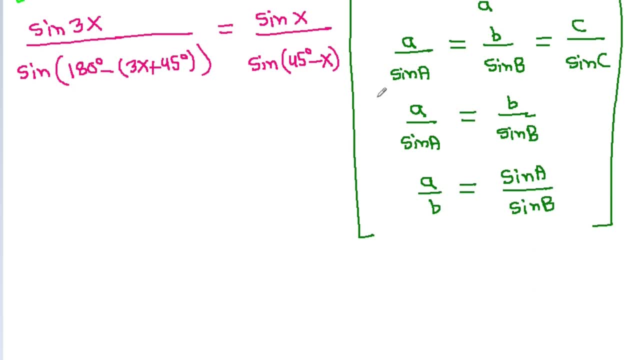 and beta is 45 degree minus x. Okay, So this is the equation, Okay, And sin 180 degree minus theta is equal to sin theta. So it is sin 3x by sin 3x plus 45 degree is equal to sin theta. 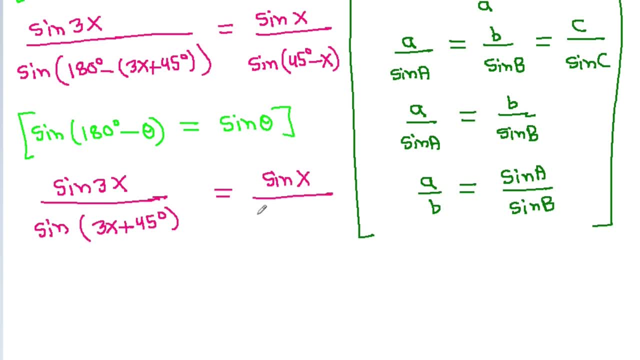 Okay, So it is sin 3x by sin 45 degree minus x, And if we cross multiply, then sin 3x times sin 45 degree minus x will be equal to sin 3x plus 45 degree minus sin theta. 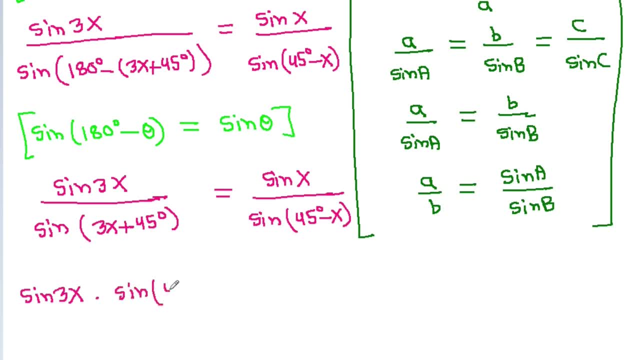 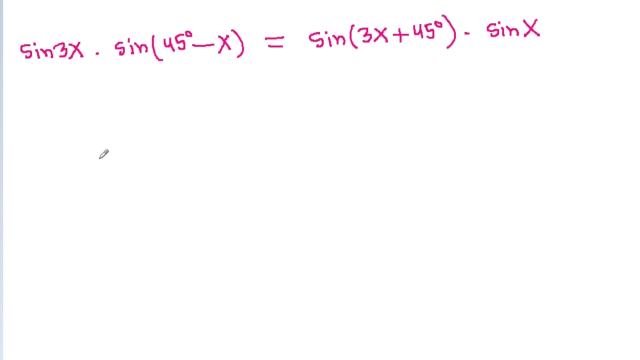 x. So it is sin 3x times sin 45 degree minus x will be equal to sin 3x plus 45 degree times sin x. And if we multiply by 2, then 2 times sin 3x times sin 3x is equal to sin 3x plus 45 degree. 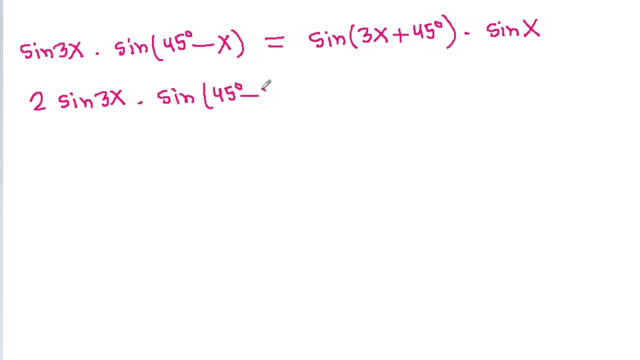 minus x. So it is sin 3x times sin 3x plus 45 degree times sin x and 2 sin a sin b, it is equal to cos a minus b minus sin x, Thank you. minus cos A plus B, So this will be cos 3x minus 45 degree, minus x, minus cos 3x plus. 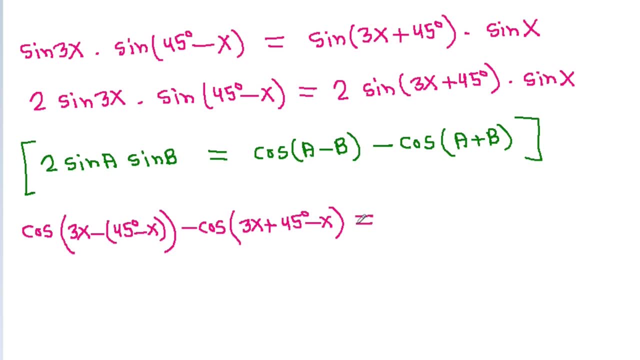 45 degree minus x is equal to: and this will be cos 3x plus 45 degree minus x, minus cos 3x plus 45 degree minus x, And it is cos 3x 3x plus x is 4x minus 45 degree minus cos. 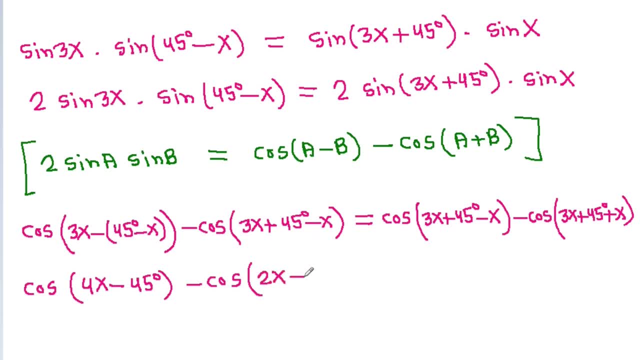 3x minus x is 2x minus 45 degree is equal to cos 2x minus 45 degree minus cos 3x plus x is 4x minus 45.. 45 degree and it is cos 4x minus 45 degree plus cos 4x plus 45 degree is equal to and. 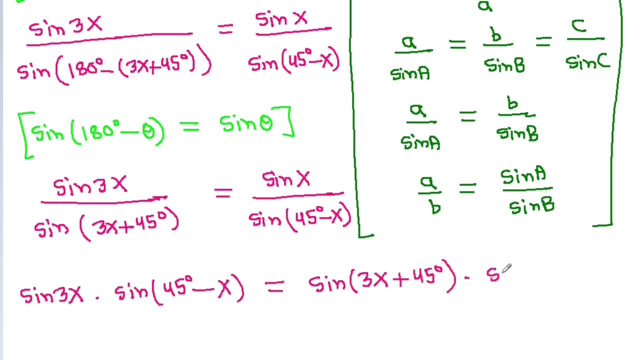 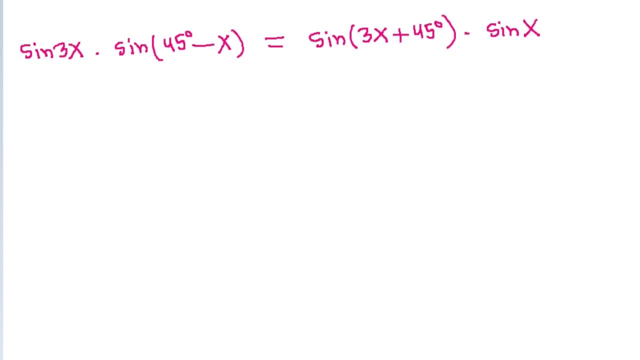 Okay, Okay, Good times. sin x, and if we multiply by 2, then 2 times sin, 3x, times sin 45 degree minus x, will be equal to 2 times sin 3x plus 45 degree times sin x and 2 sin a sin b, it is equal to. 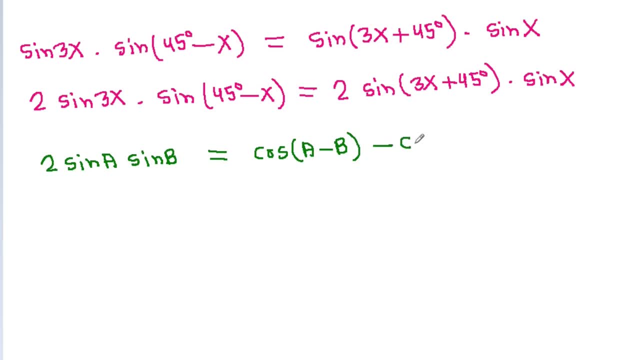 cos a minus b minus cos a plus b. so this will be cos 3x minus 45 degree minus x minus cos 3x plus 45 degree minus x is equal to: and this will be cos 3x plus 45 degree minus x minus cos 3x plus 45 degree minus x. 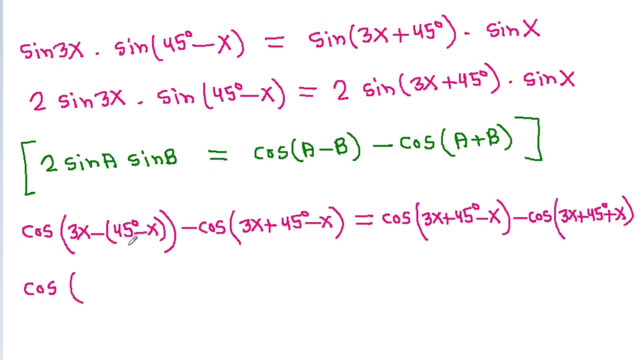 and it is: cos 3x plus x is 4x minus 45 degree minus cos 3x minus x is 2x. plus 45 degree is equal to cos 2x minus 45 degree. minus cos 3x plus x is 4x. 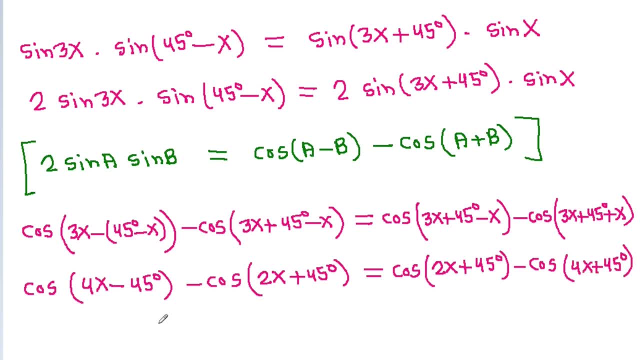 minus 45 degree, and it is cos cos 4x minus 45 degree. plus cos 4x plus 45 degree is equal to: and cos 2x minus 45 degree plus cos 2x plus 45 degree will be 2 times cos 2x minus 45 degree, and 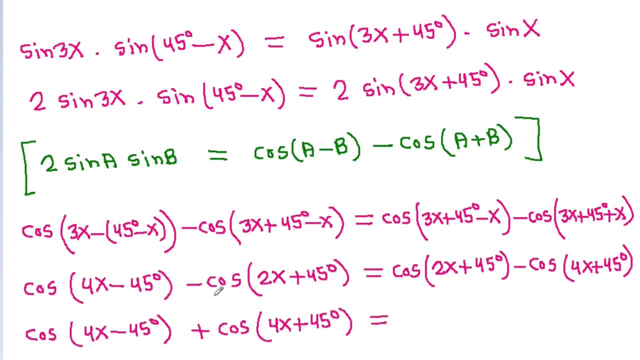 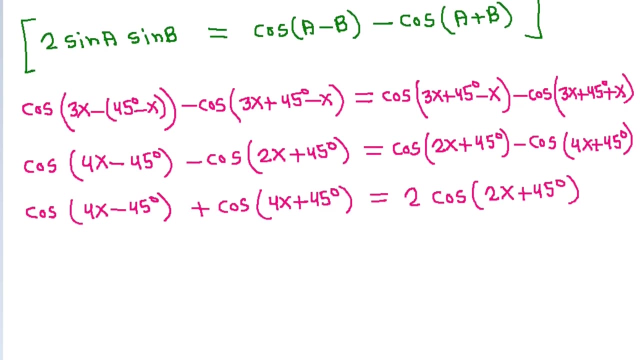 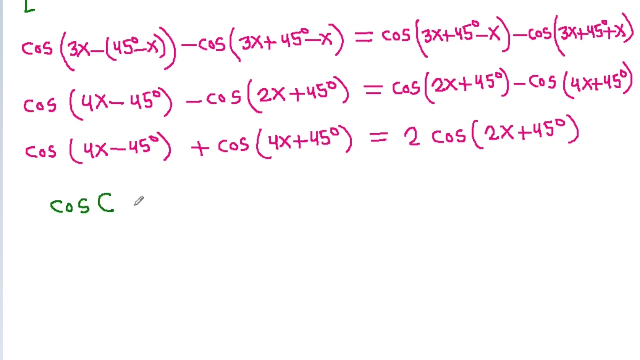 cos 2x plus 45 degree plus cos 2x plus 45 degree will be 2 times cos 2x plus 45 degree. and, and cos c plus cos d, it is equal to 2 times cos c plus d by 2, cos c minus d by 2. and cos a plus b, it is equal to cos a, cos b minus sin a, sin b. 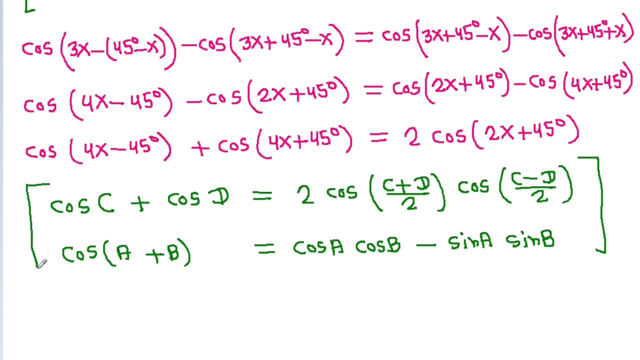 So cos 4x minus 45 degree plus cos 4x plus 45 degree will be 2 times cos, and 4x minus 45 degree plus 4x minus 45 degree by 2 will be 4x. So cos 4x minus 45 degree will do私 plus 2012 times cos, and cos 2 is equal to 2 times and 4x plus 45. 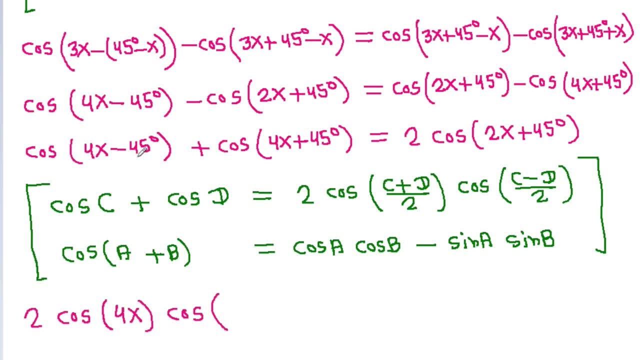 degree minus 4x. minus 45 degree by 2 would be 4x. 4x minus 45 degree is equal to 2 times, and cos 2x plus 45 degree will be cos 2x. cos 45 degree minus sin a, sin b. 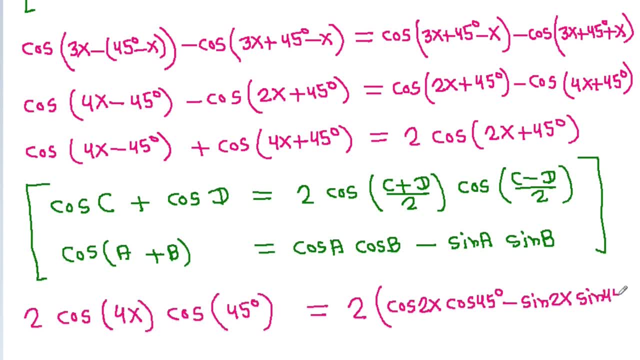 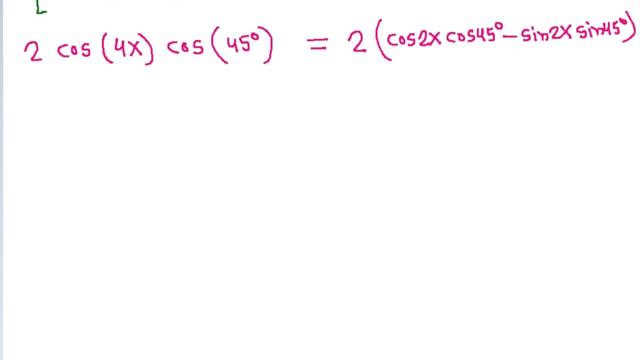 2x, sin 45 degree and 2 will get constrained and cos 45 degree will get constrained because cos 45 degree is equal to sin 45 degree. So we get: cos 4x is equal to cos 2x minus sin 2x and it is sin 2x is equal to cos 2x. 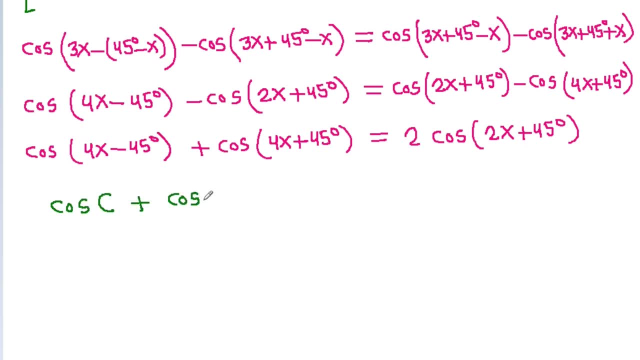 cos c plus cos d, it is equal to 2 times cos, cos c plus d by 2, cos c minus d by 2 and cos a plus b, it is equal to cos a, cos b minus sin a, sin b. so cos 4x minus 45 degree plus cos 4x plus 45 degree will be 2 times cos. 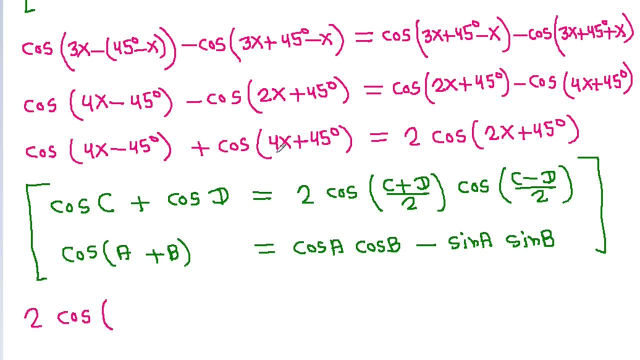 and 4x minus 45 degree minus 4x minus 45 degree by 2 will be 4x times cos times cos. and 4x plus 45 degree minus 4x minus 45 degree by 2 will be 45 degree is equal to 2 times. 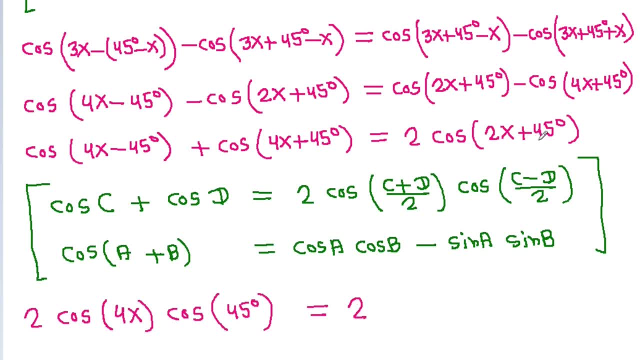 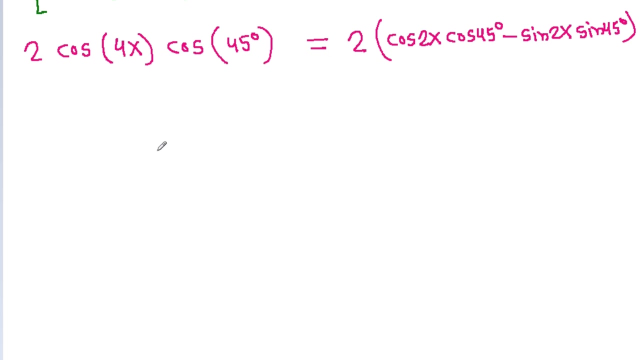 and cos 2x minus 45 degree will be cos 2x, cos 45 degree minus sin 2x, sin 45 degree and 2 will get constant. and cos 45 degree will get constant because cos 45 degree is equal to sin 45 degree. 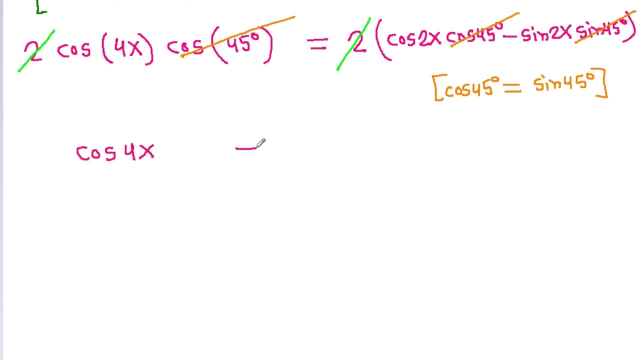 so we get: cos 4x is equal to cos 2x minus sin 2x and it is sin two. x is equal to cos 2x minus cos 4x and sin 2a is equal to 2 sin a cos a. 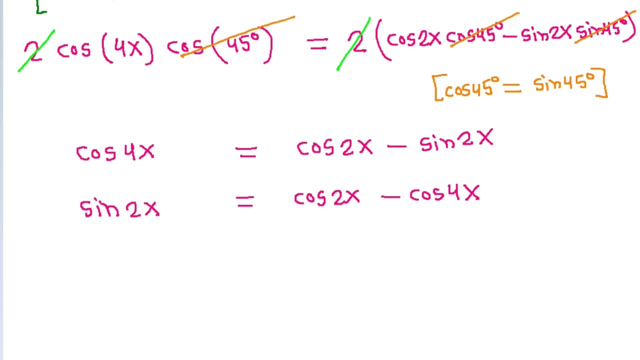 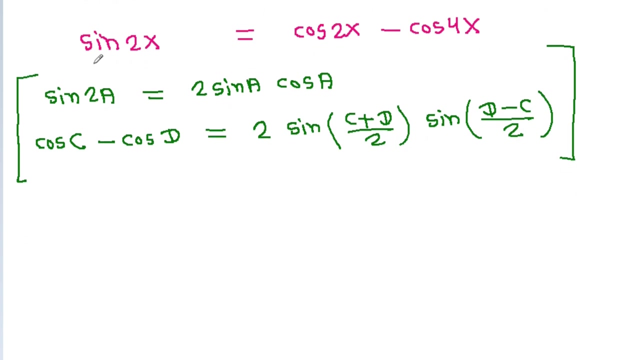 minus cos 4x, and sin 2a is equal to 2 sin a, cos a and cos c minus cos d. it is equal to 2 times sin c plus d by 2 sin 2x minus cos 4x, So sin 2x will be 2 sin x, cos x is equal to, and cos 2x minus cos 4x will be 2 times. 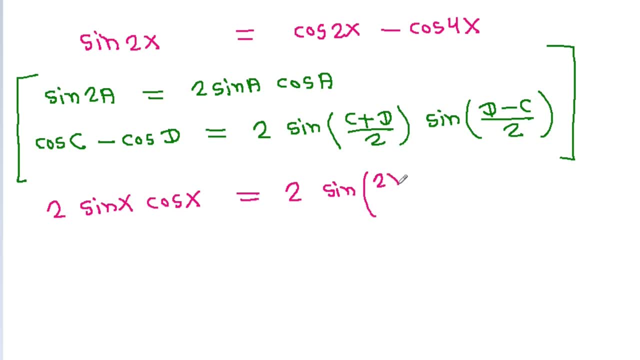 sin 2x, So sin 2x will be 2 sin x, cos x is equal to, and cos 2x minus cos 4x will be 2 times sin 2x plus 4x by 2, times sin 4x minus 2x by 2, and it is 2 sin x. cos x is equal to 2. 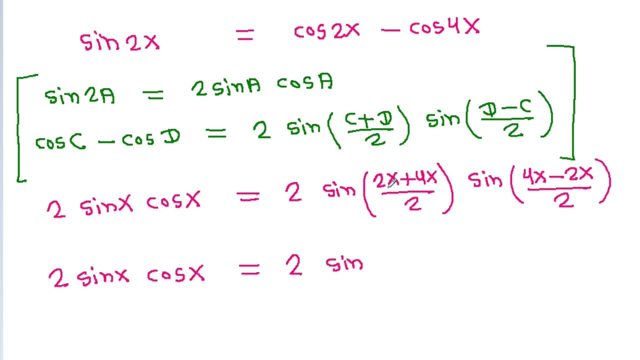 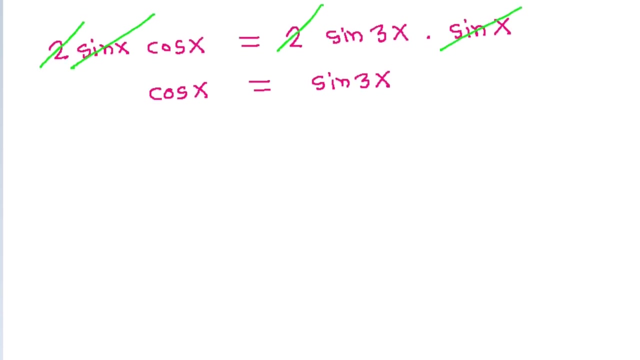 times sin 6x by 2 is 3x, So sin 2x by 2 is x and 2 will get constrained and sin x will get constrained. So we get cos x is equal to sin 3x and cos x is equal to sin 4x minus sin 4x. 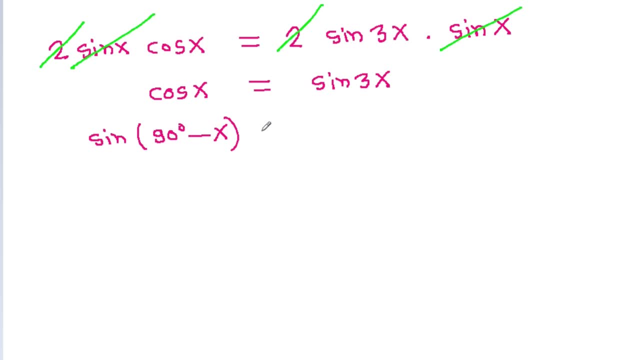 So we get: cos x is equal to sin 3x. 90 degree minus x is equal to sin 3x. So we get: 90 degree minus x is equal to 3x, and 3x plus x will be 4x is equal to 90 degree. So x is equal to 90 degree. by 4 that means x is. 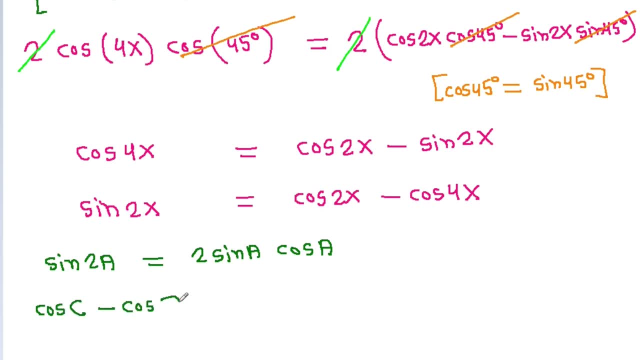 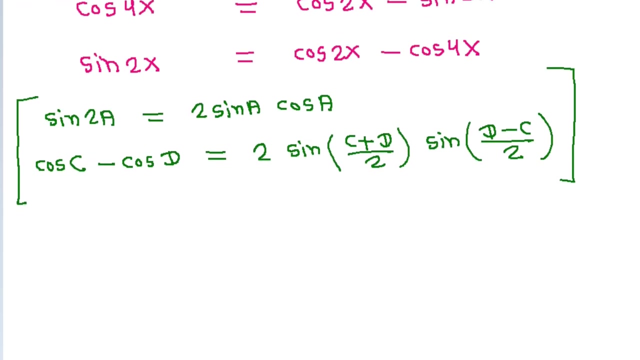 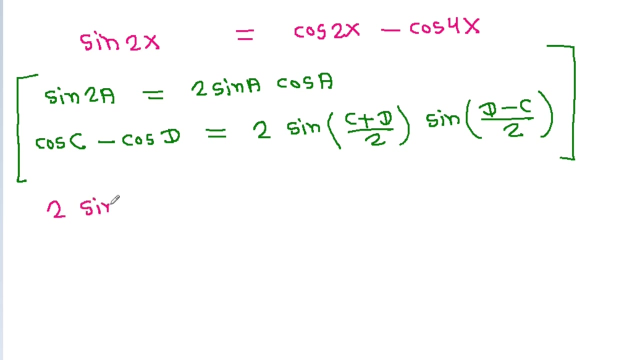 and cos c minus cos d equal to 2 times sin c plus d by 2 times sin d minus c by 2.. So sin 2x will be 2, sin x, cos x is equal to, and cos 2x minus cos 4x will be 2 times sin 2x plus 4x by 2 times sin. 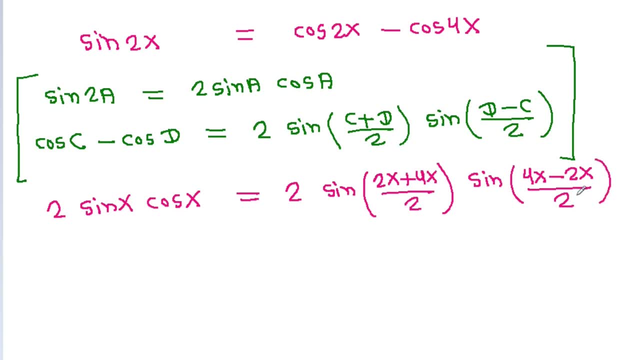 4x minus 2x by 2 and it is 2 sin x. cos x is equal to 2 times sin 6x by 2 is 3x times sin 2x by 2 is x and 2 will get cancelled and sin x will get cancelled. 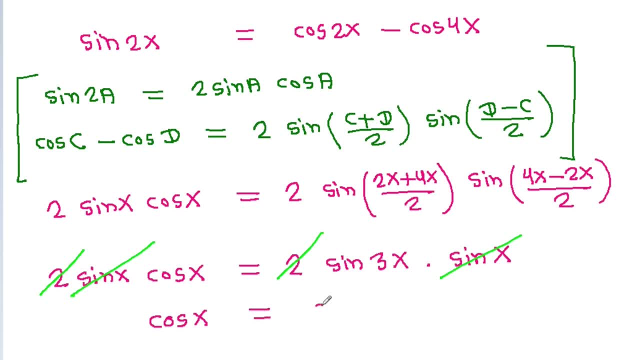 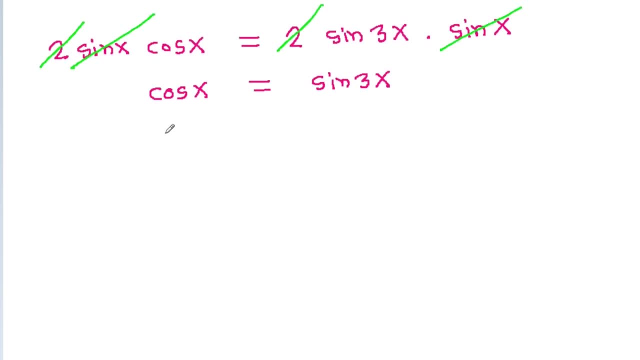 So we get: cos x is equal to sin 3x and cos x is equal to sin. 90 degree minus x is equal to sin 3x. So we get: 90 degree minus x is equal to 3x, and 3x plus x will be 4x. 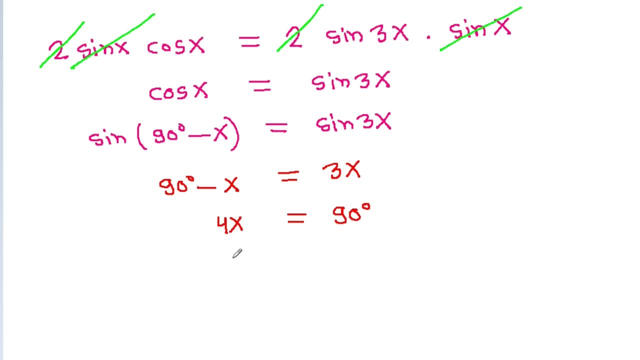 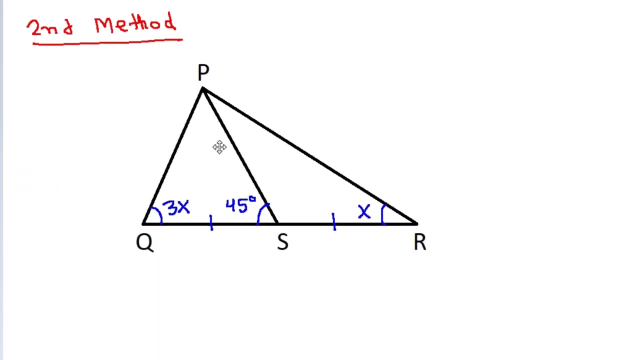 x is equal to 90 degree, so x is equal to 90 degree by 4. that means x is equal to 22.5 angle. and this second method, here this angle is alpha and this angle is beta, and we have alpha minus 3x. minus 45 degree is equal to 180 degree. that means 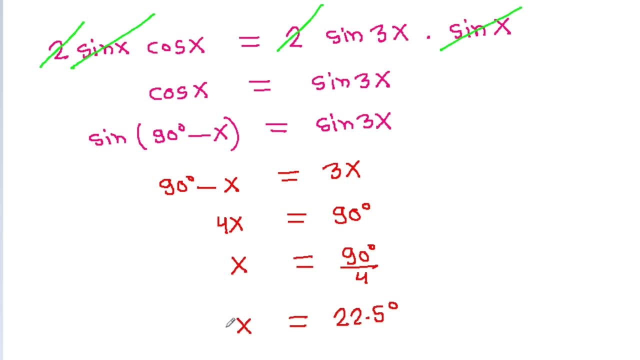 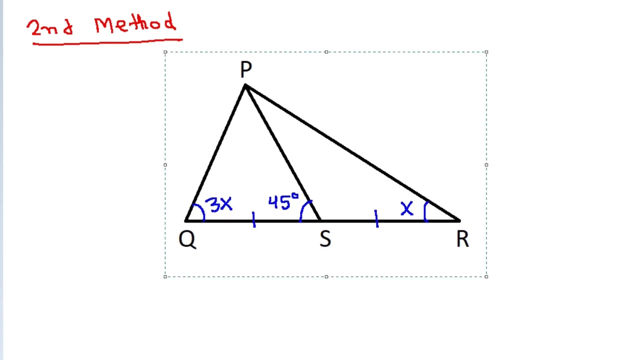 equal to 22.5 degree. and this second method: here this angle is alpha and this angle is beta and we have alpha minus 3x. minus 45 degree is equal to 180 degree. that means alpha minus 3x is equal to 135 degree. 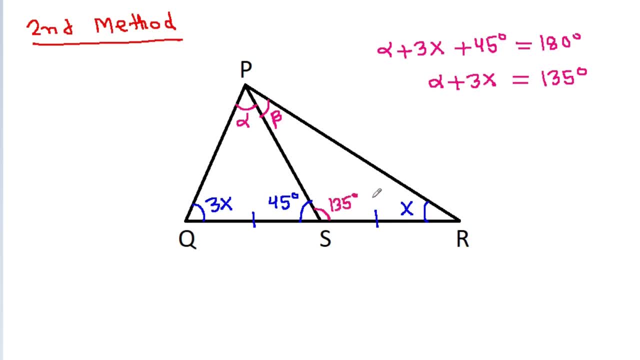 and this angle is 135 degree. So beta plus 135 degree plus x is equal to 180 degree. and beta plus x is equal to 180 degree minus 135 degree will be 45 degree, And if we multiply by 3, then 3beta plus 3x will be equal to 135 degree and from these two equations we get anpa plus. 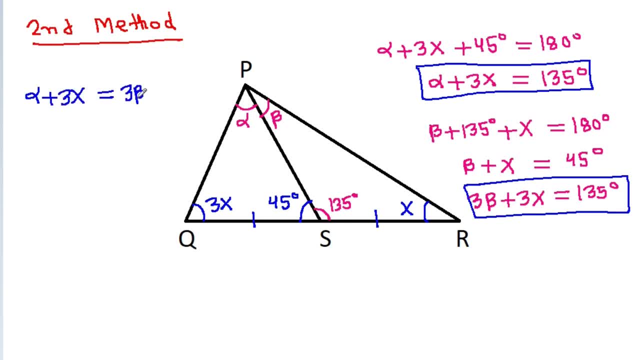 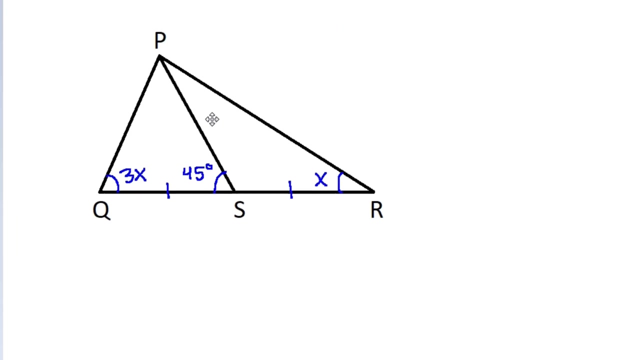 3x is equal to 3beta plus 3x, and 3x will get cancelled. so anpa is equal to 3beta and if we draw qm and join ms such that this angle is x, then this angle will be 2x and 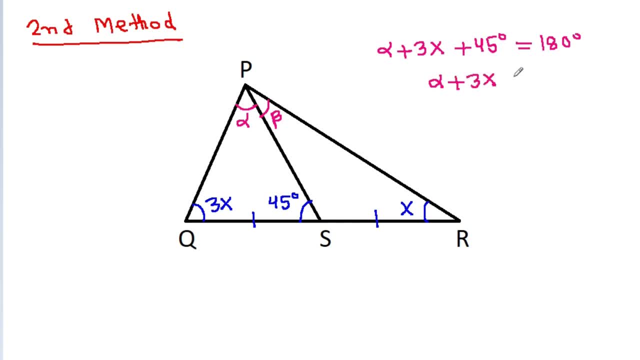 alpha minus 3x is equal to 135 degree and this angle is 135 degree. so beta plus 135 degree plus x is equal to 180 degree. and beta plus x is equal to 180 degree minus 135 degree will be 45 degree. and if we multiply by 3, then 3 beta plus 3x will be equal to 135. 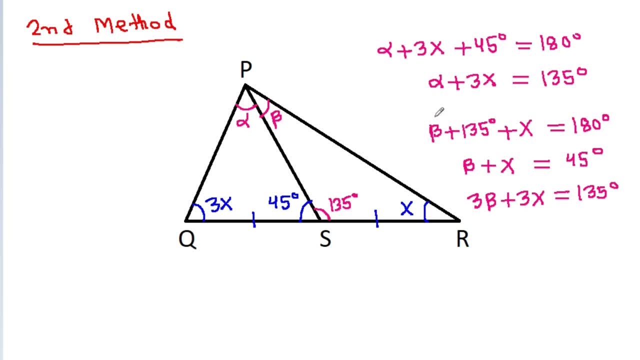 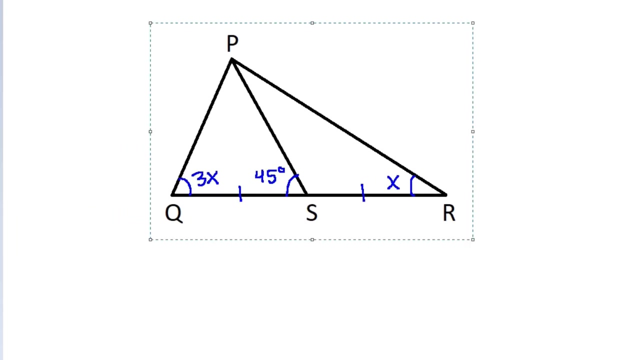 degree and from these two equations we get: alpha plus 3x is equal to 3 beta plus 3x, and 3x will get cancelled. so alpha is equal to 3 beta plus 3x is equal to 3 beta plus 3x. and if we draw, 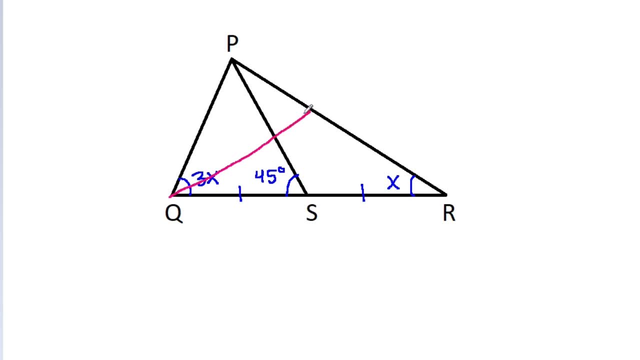 qm and join ms such that this angle is x, then this angle will be 2x. and in triangle QMR, this is Q, this is M and this is R and this is S and this angle is X, this angle is X. That means triangle QMR is isosynous. 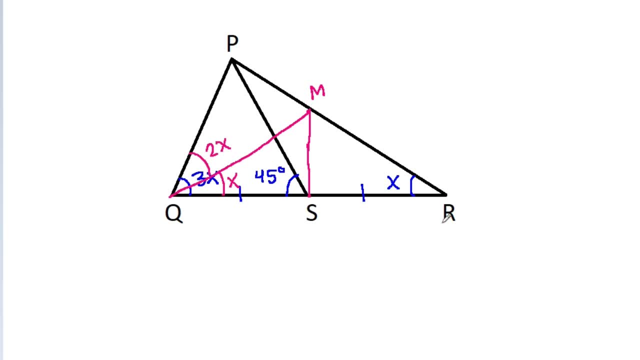 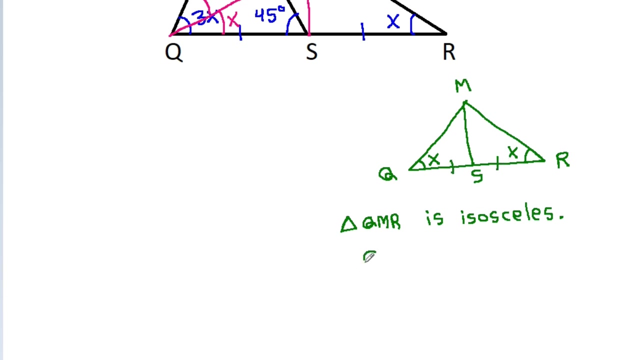 in triangle qm are: this is q, this is m and this is r and this is x and this angle is x. that means triangle qm, r is isosinus and also Qs is equal to Sr. Qs is equal to Sr, it is given. that means angle. Qsm will be 90 degree. 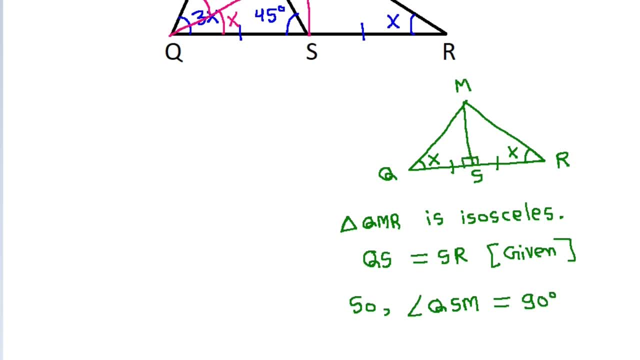 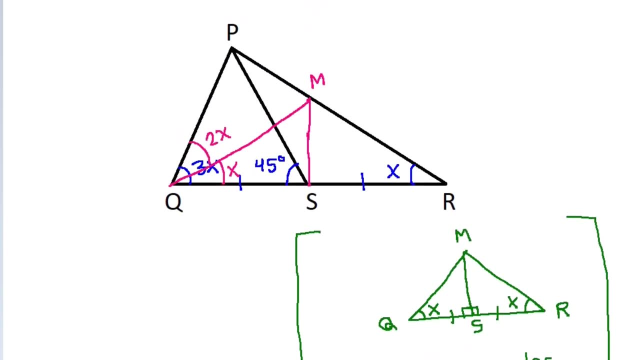 this angle will be 90 degree. so this angle is 90 degree. that means this angle will be 45 degree and in any triangle, if this angle is A, this angle is B, then this angle it is A plus B. 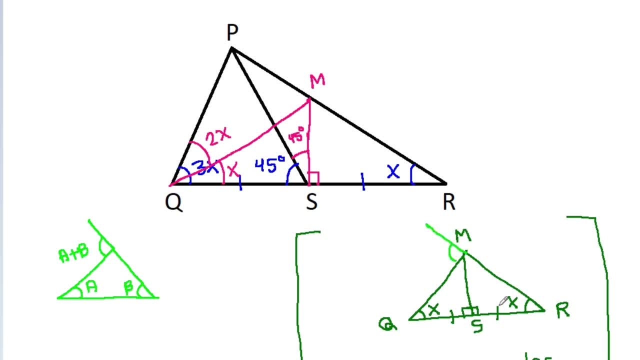 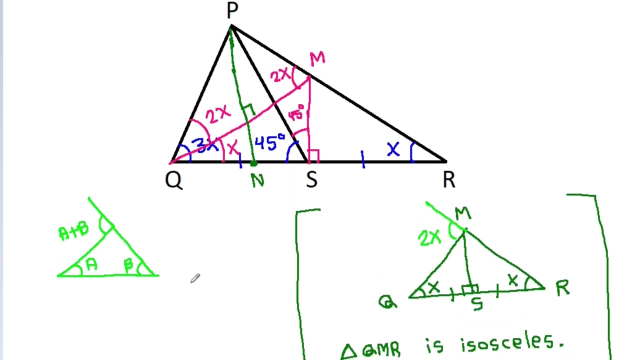 so this angle, it will be x plus x, that is 2x. so this angle is 2x. and if we draw a perpendicular from P, this is right angle. and suppose this point is N, then in triangle PQM. 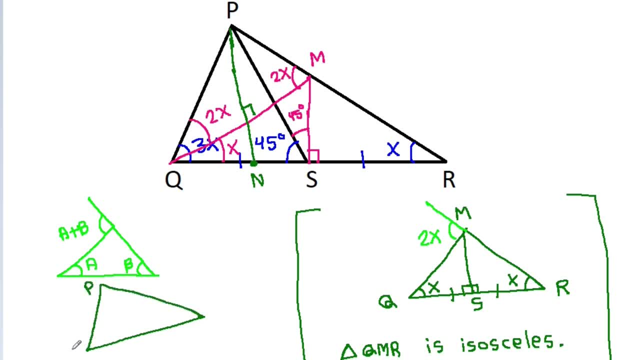 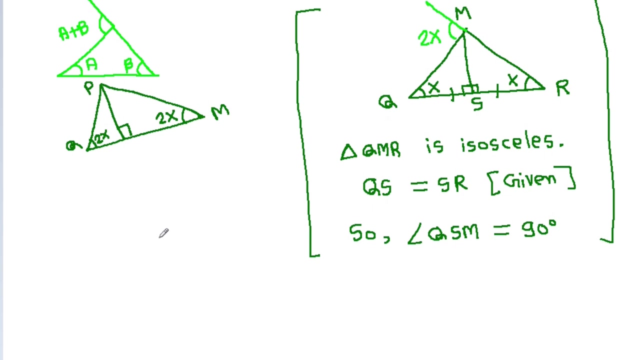 this is PQM and this is right angle. and this angle is 2x and this angle is 2x and in any isosyncrt triangle, if these two angles are equal, if these two angles are equal, and this is perpendicular. 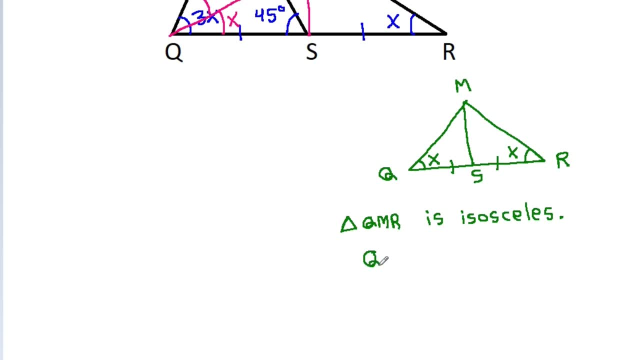 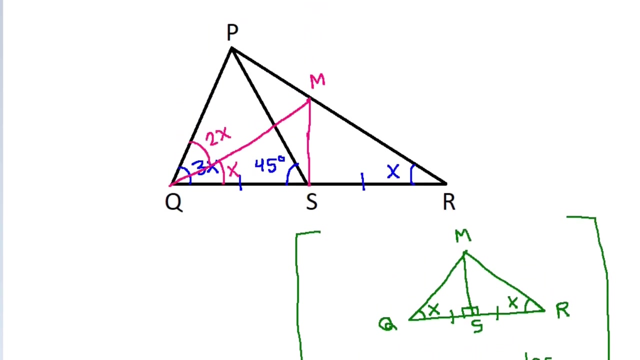 and also QS is equal to SR. QS is equal to SR. it is given: Okay, That means angle: QSM will be 90 degree. this angle will be 90 degree. So this angle is 90 degree. that means this angle will be 45 degree. 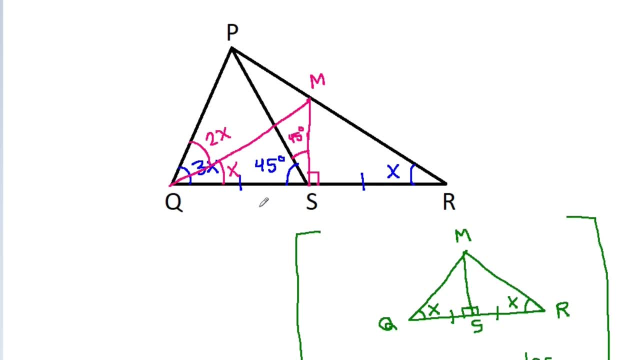 Okay, And in any triangle, if this angle is A, this angle is B, then this angle it is A plus B. So this angle, it will be X plus X, that is 2x. Okay, So this angle is 2x. 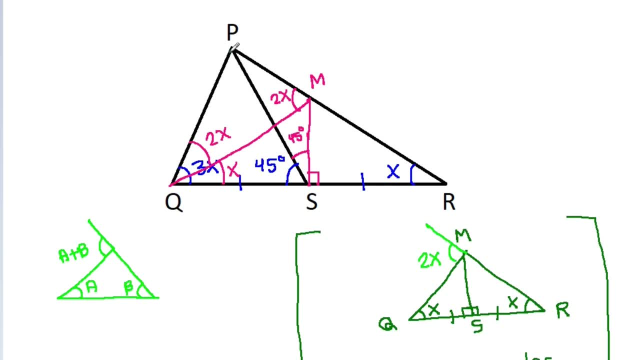 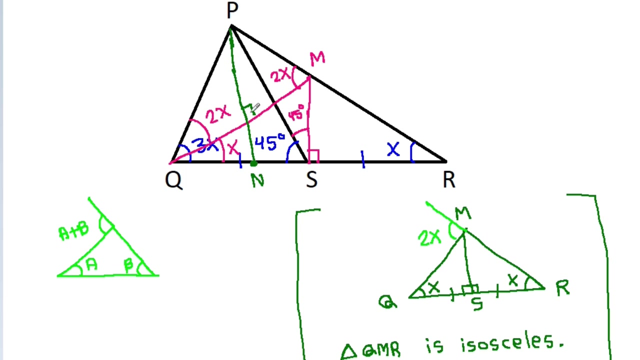 And if we draw a perpendicular from P, this is right angle and suppose this point is N in triangle PQM. this is PQM and this is right angle and this angle is 2x and this angle is 2x. Okay, 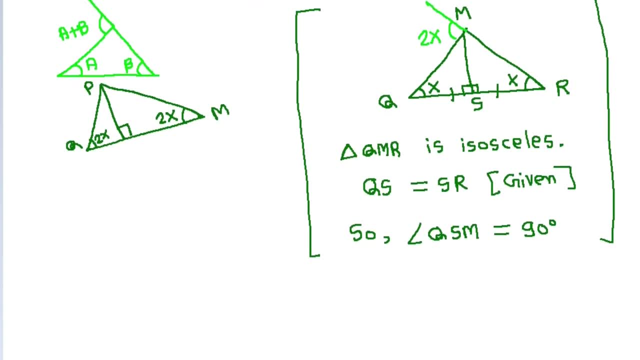 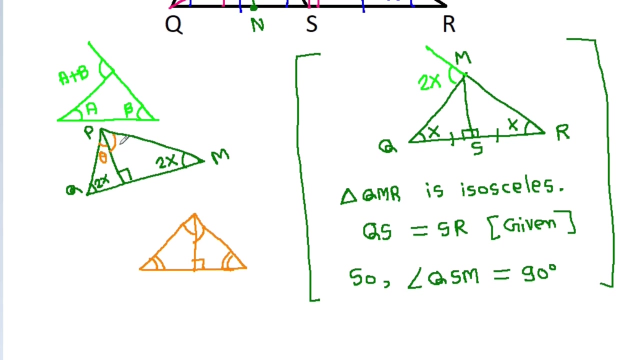 Okay, Okay, Okay, Okay. And in any isosynous triangle, if these two angles are equal- and this is perpendicular- then these two angles will be also equal. That means, if this angle is theta, then this angle will be theta. 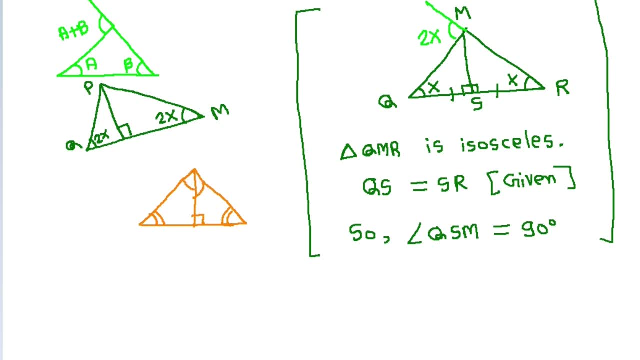 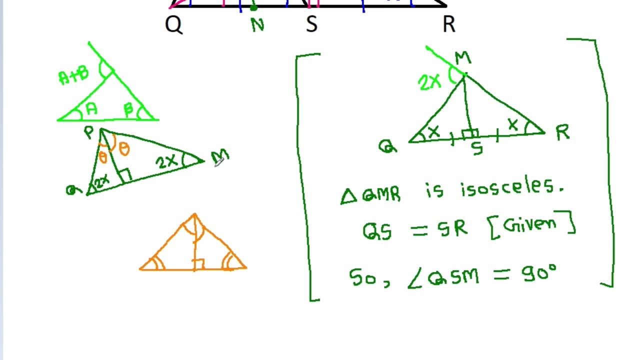 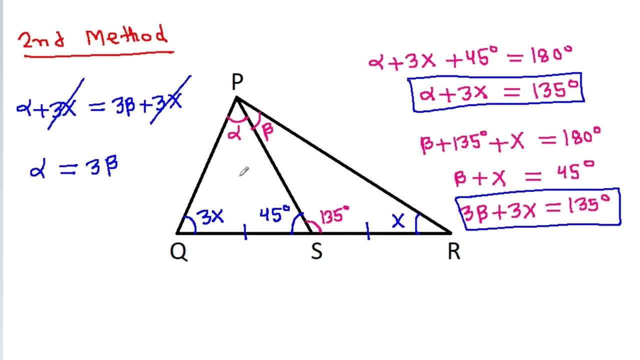 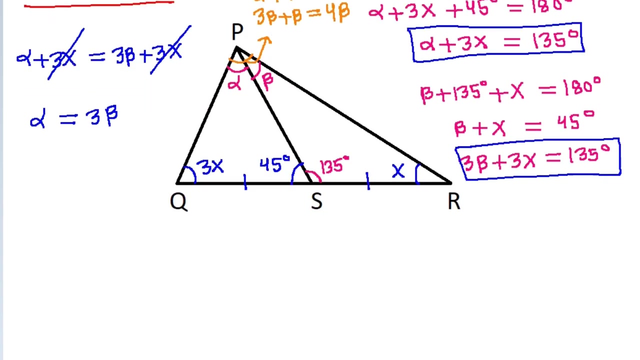 then these two angles will be also equal. that means, if this angle is theta, then this angle will be theta. and here we have this angle. it is alpha plus beta, and alpha is 3 beta plus beta, that is 4 beta. 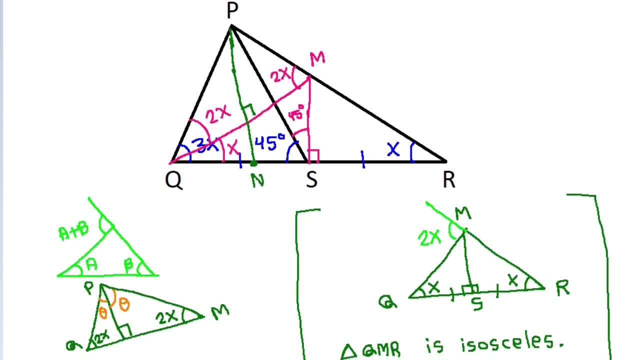 and that means theta plus theta is equal to 4 beta, so theta will be equal to 2 beta. so this angle is theta, that is 2 beta, and this angle is beta, so this angle will be beta. 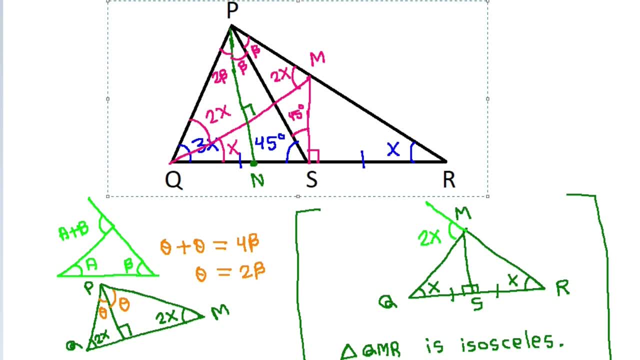 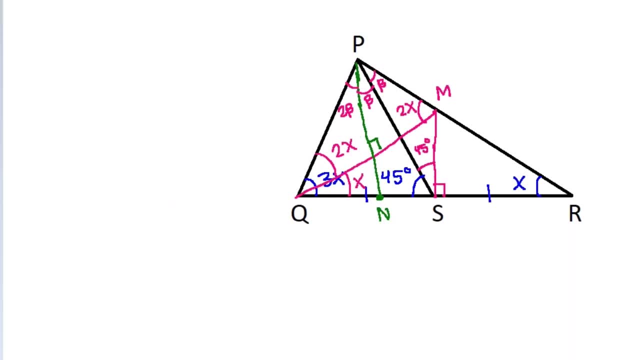 and now in triangle P in S and triangle P, M S. here this is P, this is N, this is S and this is M, and these angles are equal: beta and beta, and. 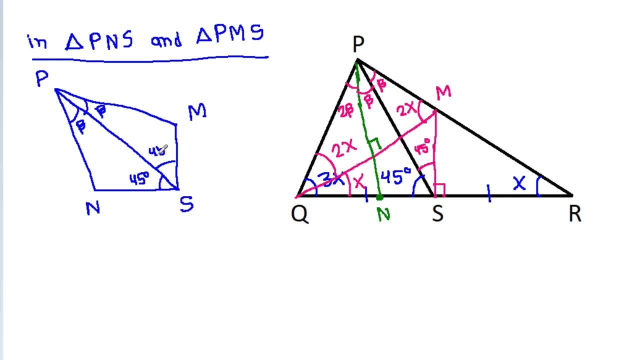 these angles are 45 degree. 45 degree and P S is common side. P S is common side. that means triangle P N S will be congruent to triangle P M S. so we get N S is equal to M S. 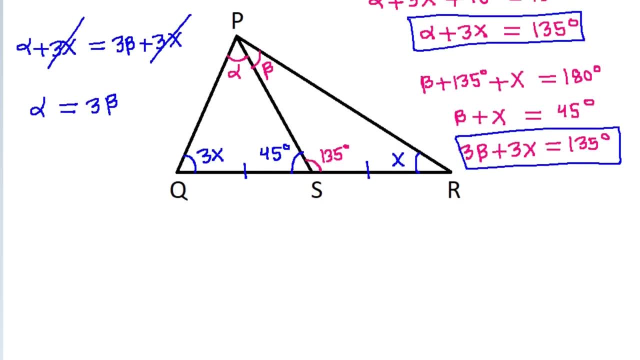 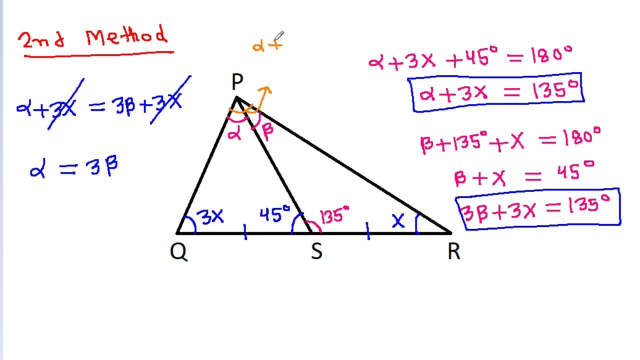 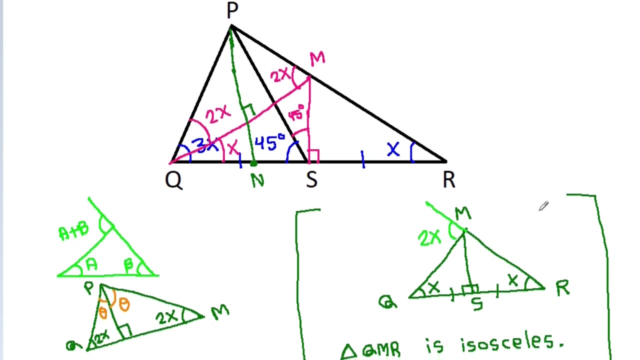 Okay, Okay, Okay, Okay. Okay, Here we have this angle. it is α plus β, and α is 3 β plus β, that is 4 β. and that means θ plus θ is equal to 4 β. so θ will be equal to 2 β. so this angle is θ, that is 2 β. 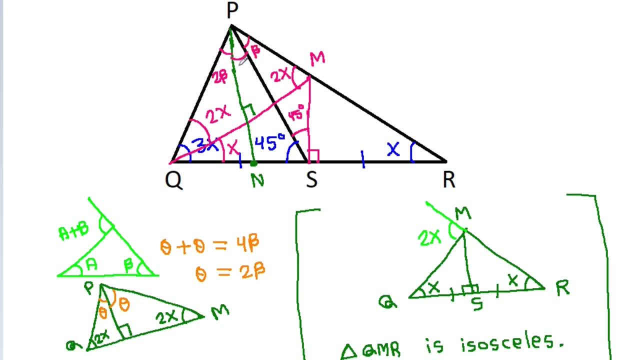 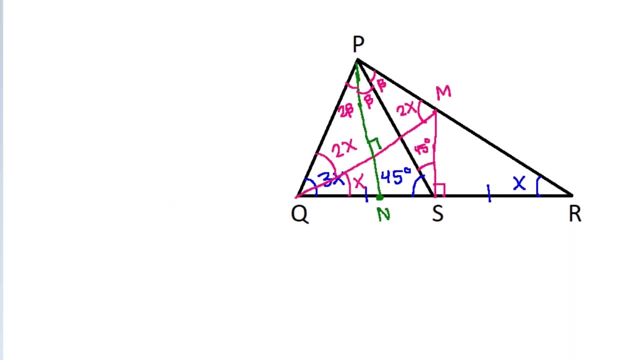 and this angle is β, so this angle will be β. and now in triangle P N S and triangle P M S: here this is P, this is N, this is S and this is M, and these angles are equal: β and β. 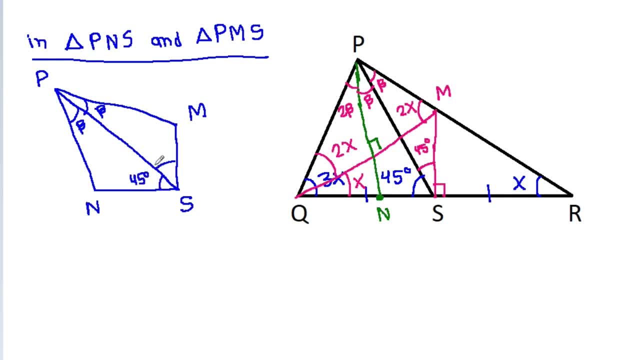 and these angles are 45, 45 degree. 45 degree and P? S is common side. P S is common side. that means triangle P N S will be congruent to triangle P M S, so we get N? S. 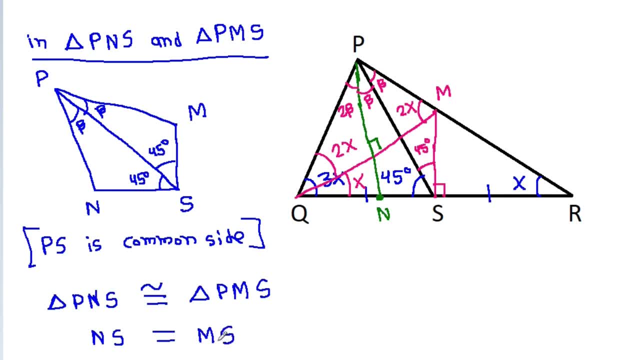 is equals to angle P, S. that means in triangle, M, S, N. this is M, this is N and this is S. this angle is 45 plus 45, 90 degree and ns is equal to sm. So these two angles will be equal, and 45 degree. This angle is 45 degree. 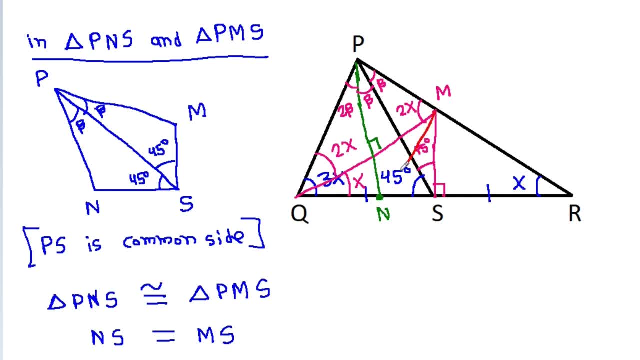 that means in triangle, M, S, N, this is M, this is N and this is S. this angle is 45 plus 45, 90 degree and N- S is equal to S, M. so these two angles will be equal and 45 degree. 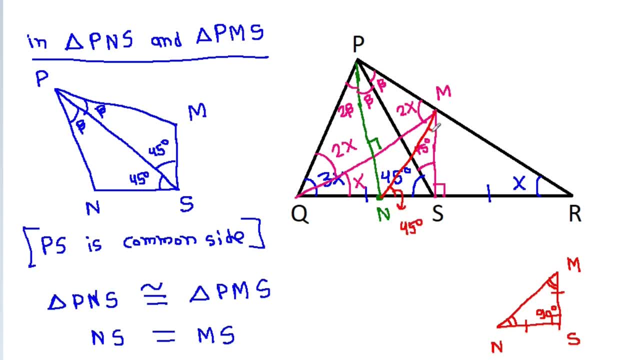 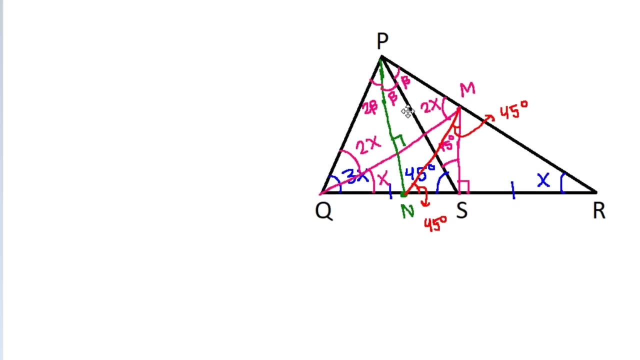 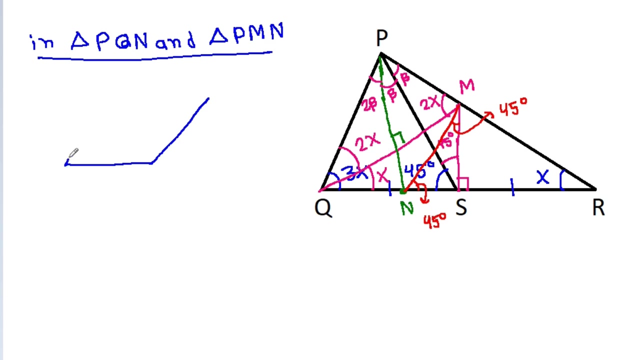 this angle is 45 degree and this angle, it is also 45 degree, also 45 degree, and now in triangle P Q N and triangle P Q M N. this is P. 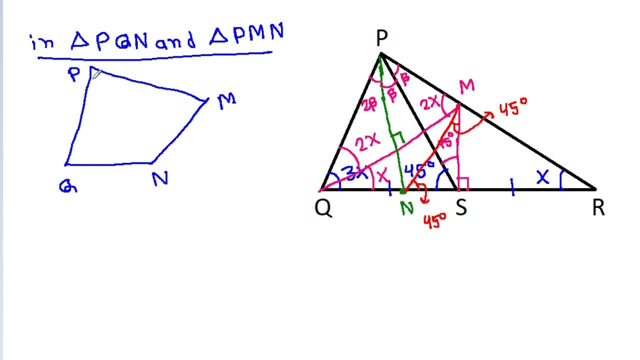 Q N M, this angle is 2 beta and this angle is beta plus beta, that is 2 beta. and in triangle P, Q M, this angle is 2x and this angle is 2x. 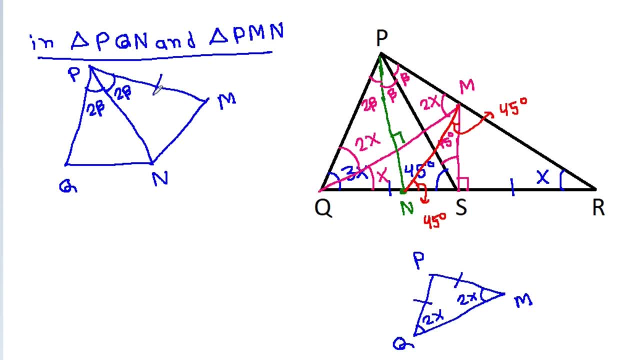 that means these two sides are equal. P M is equal to P Q and P N is common side. that means triangle Q N will be congruent to triangle P M N. that means: 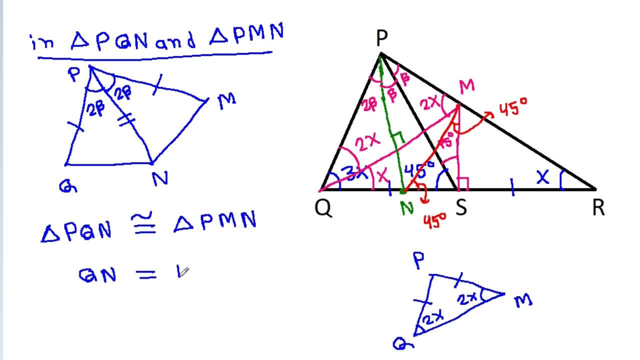 Q N is equal to M N and this is Q N M. if Q N is equal to M N, then these two angles will be equal, and this angle is x, so this angle. 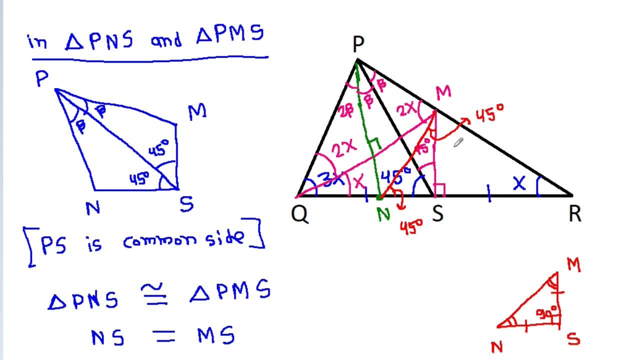 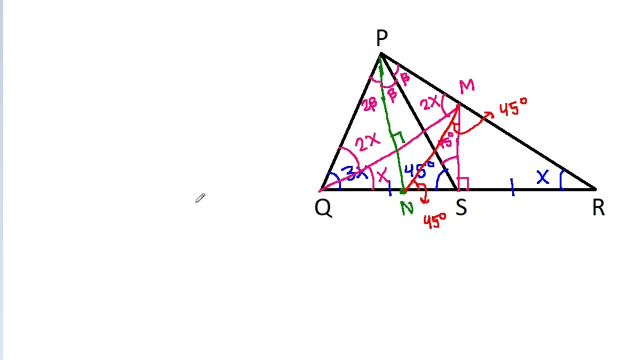 and this angle, it is also 45 degree. And now in triangle p q n and triangle p m n, this is p q n m. This angle is 2 beta and this angle is beta plus beta. that is 2 beta. 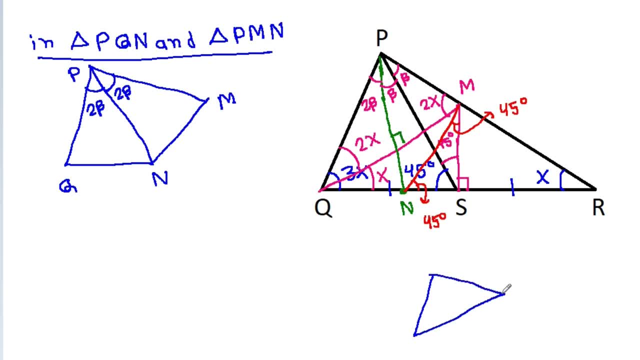 and in triangle p q m, this angle is 2x and this angle is 2x. that means these two sides are equal, p m is equal to p q and p n is common side. that means triangle p q- n will be congruent. 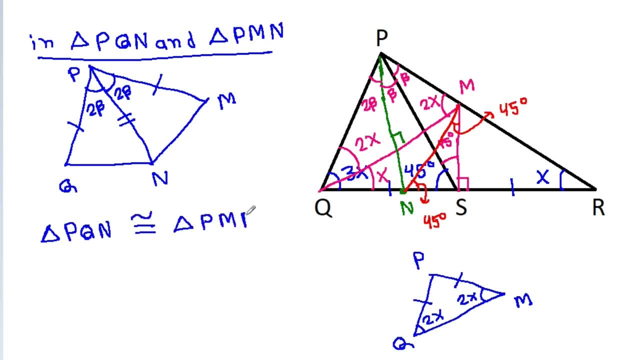 to triangle p m n. That means q n is equal to m n and this is q n m. If q n is equal to m n, then these two angles will be equal, and this angle is x, so this angle will be x. 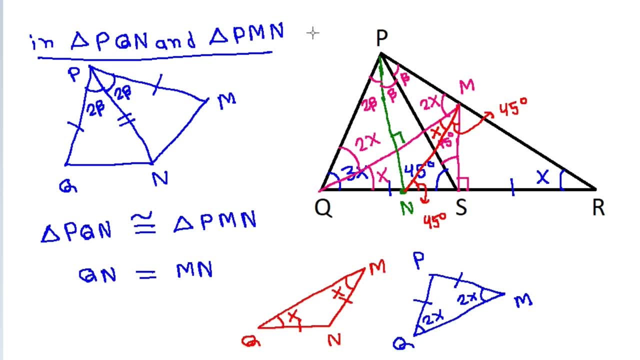 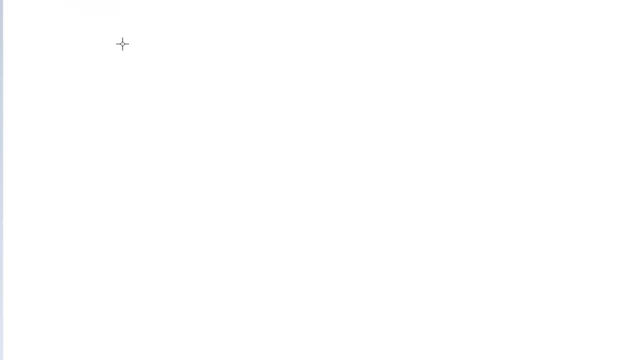 This angle will be x. And now in triangle q, m, n, this angle is x. This angle is 45 degree. This angle is x, This angle is x. So x plus x will be equal to 45 degree and 2x is equal to 45 degree.